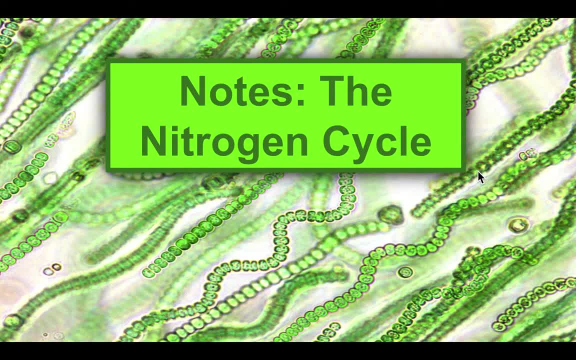 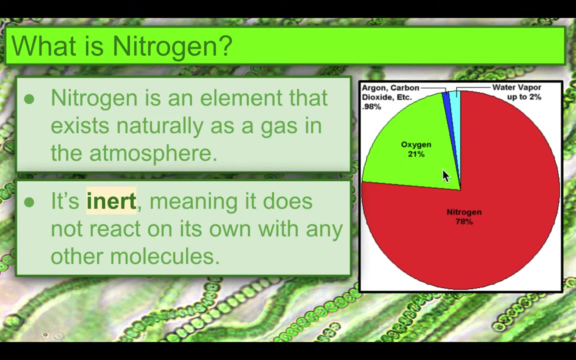 In our first virtual lecture together, we're going to go over the nitrogen cycle. So what is nitrogen? Well, it is a gas. It exists in the atmosphere And if we look at this pie chart, the majority, the vast majority of the atmosphere is nitrogen. Nitrogen is an inert gas. So what? 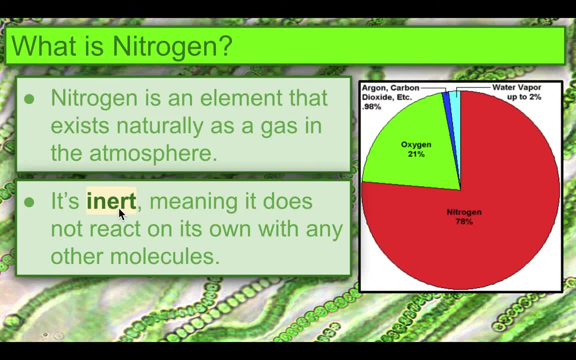 does that mean? Well, an inert gas doesn't react with other molecules, They just kind of stay to themselves, Unlike carbon, carbon is the kind of atom that likes to interact and bond and such and not so much nitrogen. Nitrogen is very much the opposite. It just likes to stay by itself. 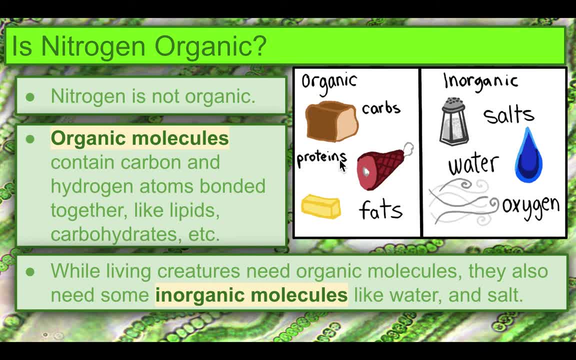 Okay, so there's two kinds of molecules in the world. There's organic and inorganic molecules, And I I, when I say this, I'm not talking about grocery store produce. That's different. Organic molecules, they just contain carbon and hydrogen atoms that are bonded together. That's it. 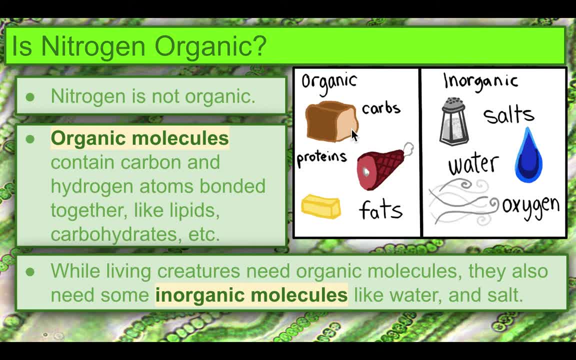 So examples are all of these here: Fats, proteins, carbohydrates, any of those macromolecules that you learned about in biology. That's all organic. And then there's inorganic molecules. These, the these inorganic molecules do not have carbon and hydrogen. 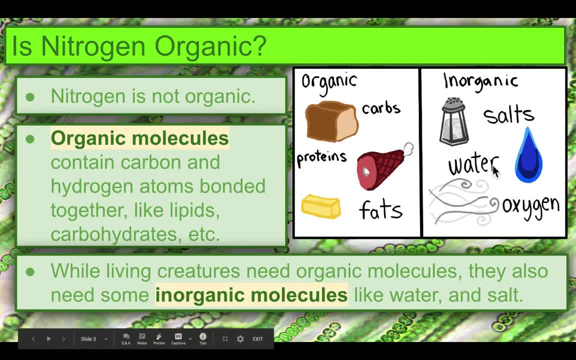 They're not organic. They're just water and hydrogen bonded together. So water has hydrogen, has two hydrogen and one oxygen, No carbon. So water is technically inorganic and it's an example of an inorganic molecule that your body must have access to and can use. So there's inorganic. 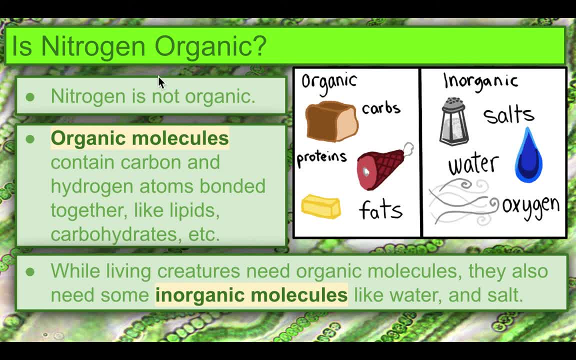 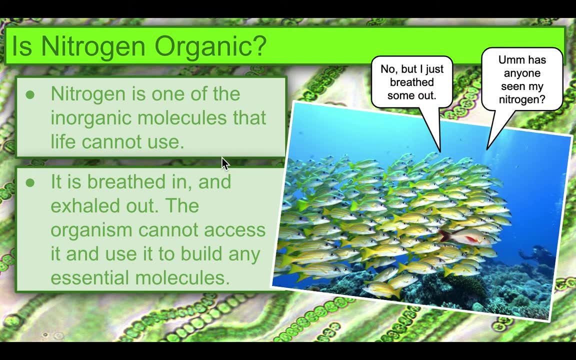 molecules your body can use, like salt. Nitrogen is an example of a molecule that is not organic, So it's inorganic. Your body cannot use it. use it, but your body needs it. So all these fish in this picture that you see, they all. 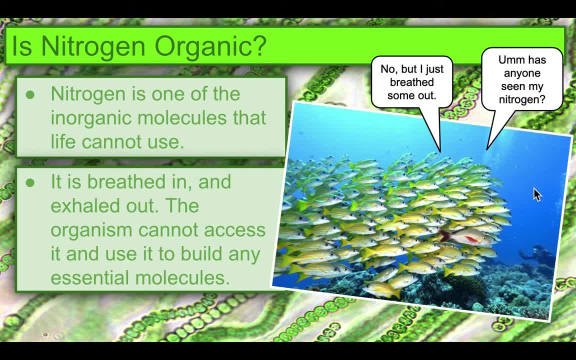 need access to nitrogen. It's dissolved in the water as a gas. It comes in through their mouth, it passes through their gills and out of the body and the nitrogen goes unused by the fish. But the scary part is all these fish need nitrogen. They need it to build. 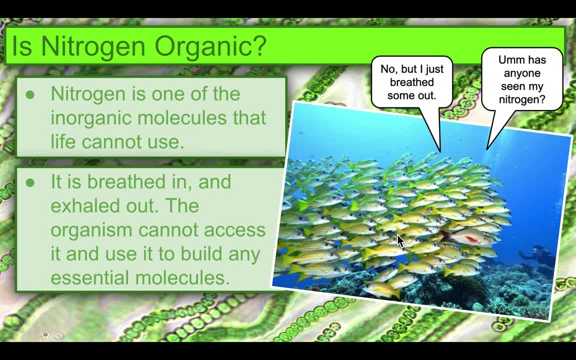 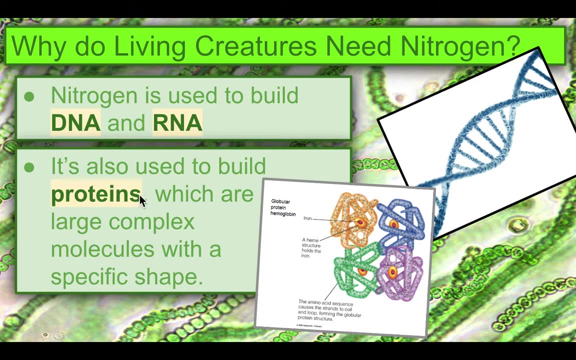 essential molecules. So this is kind of like getting pretty scary here. So how are they getting their nitrogen? I certainly hope. And what are they building? Well, they're building DNA and RNA and they're also building proteins, If you look: DNA and RNA and proteins. 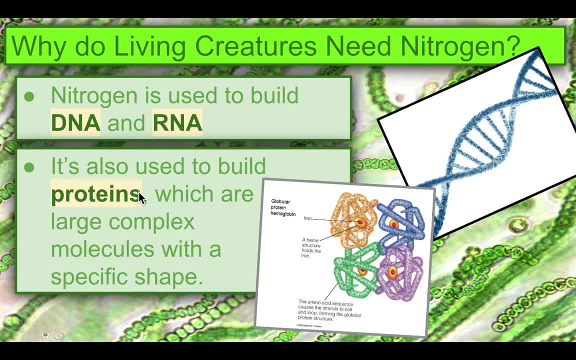 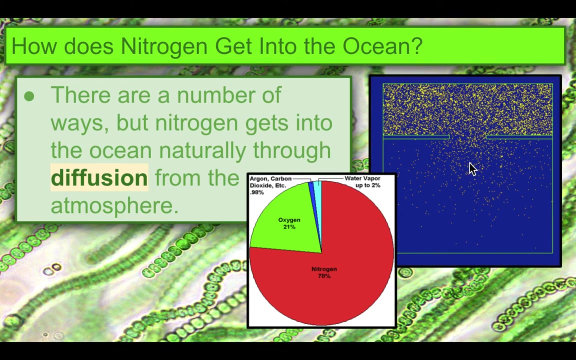 are all built with nitrogen. They're built with other atoms too, like carbon and hydrogen, because they're organic, But you know nitrogen. you can't build these without nitrogen, So this is a pretty important atom to build these things. So how does the nitrogen get into the ocean water? 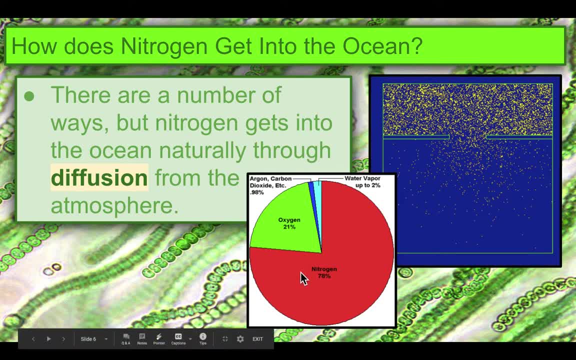 Well, there's several ways We learn. the atmosphere is mostly nitrogen, so gases that are in the atmosphere diffuse into the ocean, So they just the process of diffusion. they exist in high concentration in the atmosphere, so they go down and diffuse into the water. 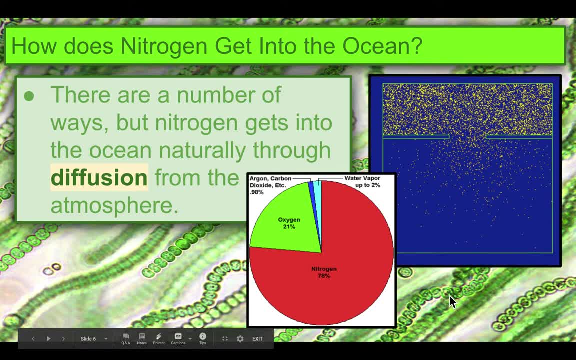 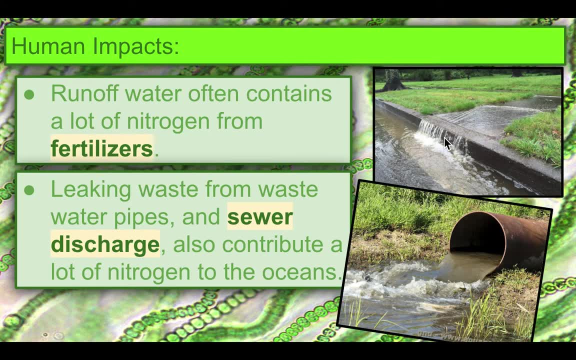 There's another way. unfortunately, that nitrogen gets into the ocean, and it's from humans. Rainwater runoff is going to contain a lot of fertilizers that plants didn't get a chance to use yet, And those runoff waters take that fertilizer straight to coastal oceans. 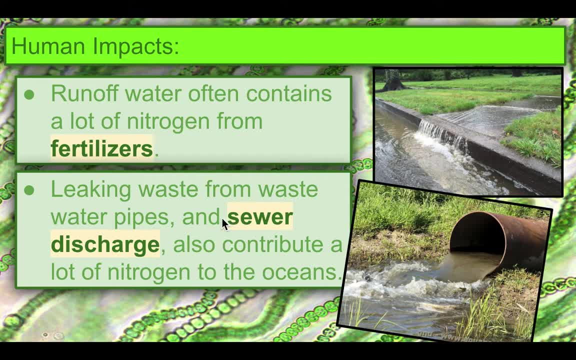 It can cause havoc on those ecosystems, irreversible damage. There's also, you know, a whole host of leaking, So there's a lot of waste water pipes and sewer discharge that takes place And that's also bringing nitrogen to the ocean. So so there's a lot of ways, unfortunately, that. 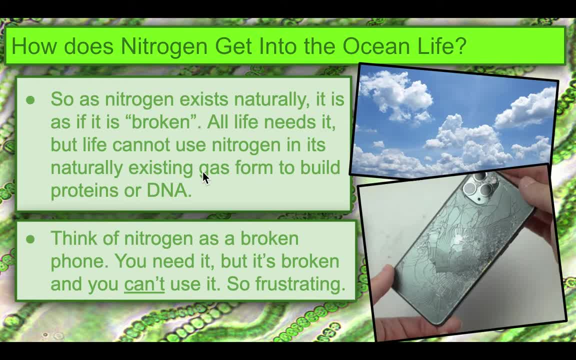 nitrogen makes its way to the ocean. OK, so the first thing that you need to know is that cell phones, when they become broken- like this unfortunate 11 here we see- it's something that you can't really use anymore because it's broken. 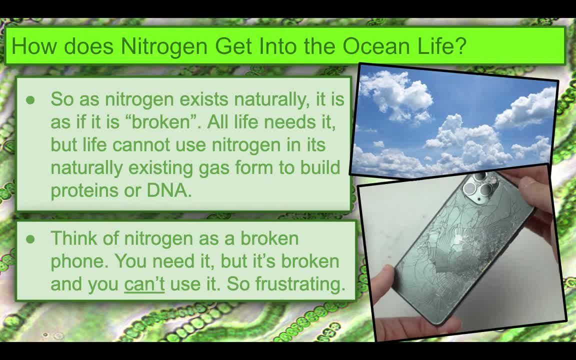 And I want you to think of nitrogen gas in that exact moment. I want you to think of nitrogen gas in that exact moment. You can't use it anymore because it's broken. And I want you to think of nitrogen gas in that exact moment. 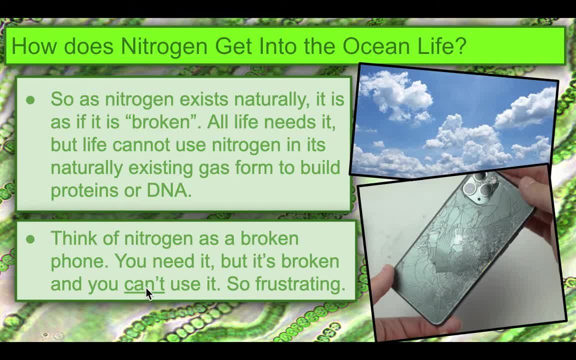 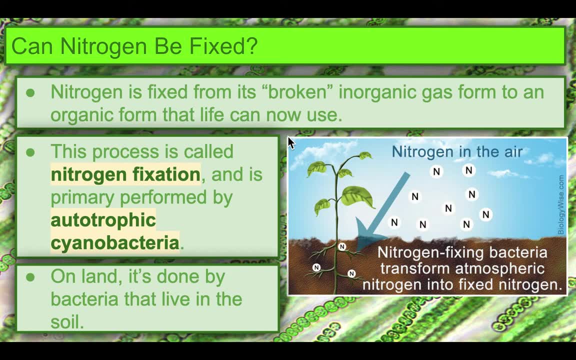 same way it's broken. you need to use it. you want to use it, but you can't because it's broken. all right, when things are broken, you can typically fix them, hopefully right. so that is why we've been thinking about nitrogen as being broken as it exists in its inorganic form, as nitrogen gas. 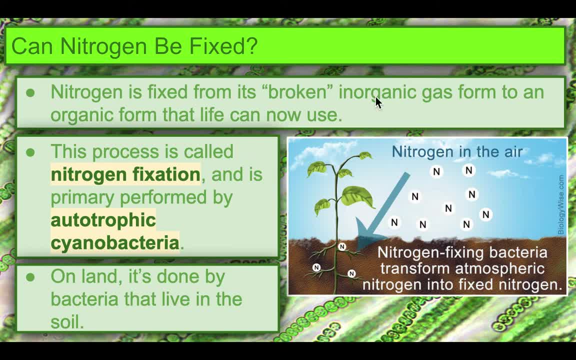 that's technically broken. so this broken inorganic gas is going to be fixed and you can see the word fix right there and this process that fixes broken nitrogen is called nitrogen fixation. so i love it. i love how it has this word fix in there. it's perfect. so that's the very beginning. 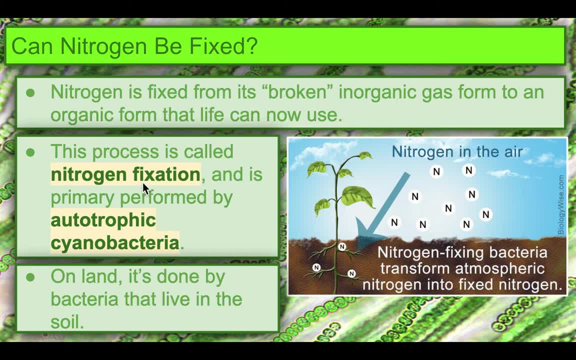 of the nitrogen cycle. its inorganic broken form is fixed right away. now, who is doing this? autotrophs. so these are animals that are animals. sorry, these are. these are plants that need access, plants and bacteria that need access to the sun. all right, so this word, cyanobacteria, that's. 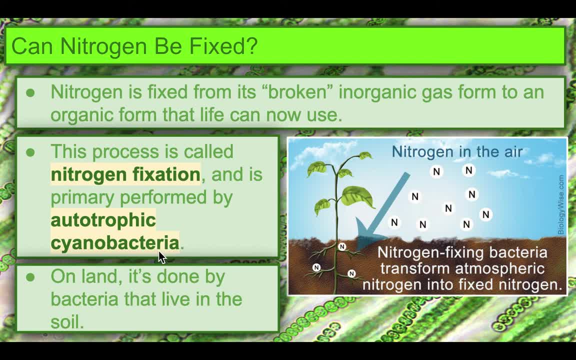 you, we can just call it bacteria, but they're also labeled as phytoplankton as well, so this is all pertaining to the ocean. but on land, this is done under the soil. that's why roots- plant roots- are under the soil, and if you rip them out of the soil, the plant typically dies. so 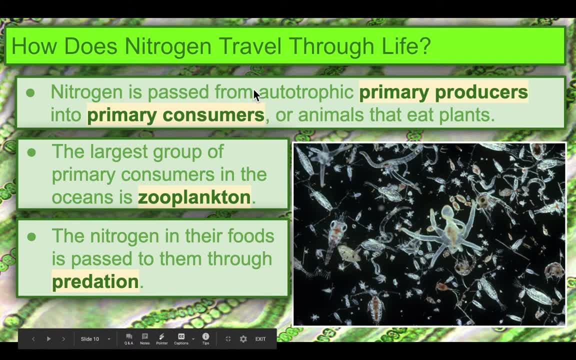 okay. so we have the fixers, Our phytoplankton, our bacteria. they fixed the broken nitrogen. It's now organic And it's going to be passed to primary consumers as they consume and eat those fixers, the bacteria and other phytoplankton. So now we 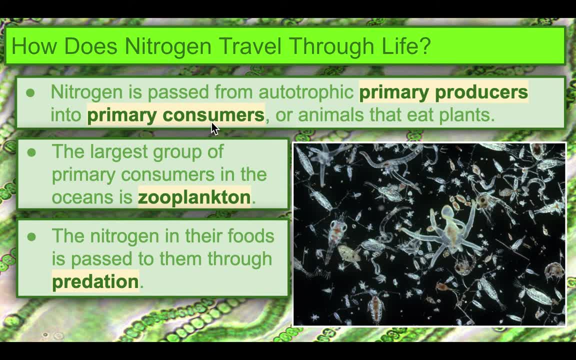 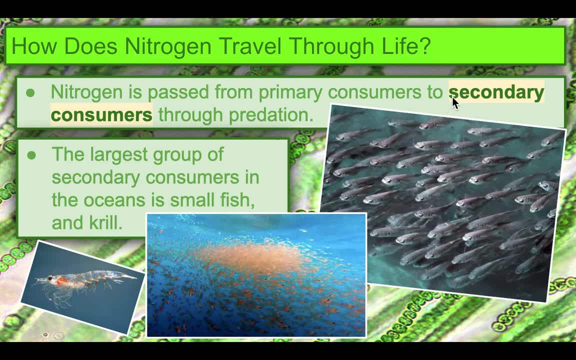 have animals that contain organic nitrogen in their bodies. They're building DNA, They're building proteins. Oh, wait a minute. They get eaten by secondary consumers. I know it's a terrible process, but this is just what happens, guys. It just happens Secondary. 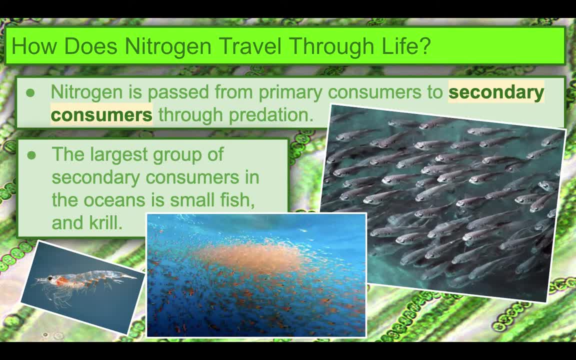 consumers get eaten by third-level consumers and third-level consumers get eaten by top-level consumers. The largest group of secondary consumers in the ocean is probably small fish and krill. and that's krill. That's literally what they look like in the water. 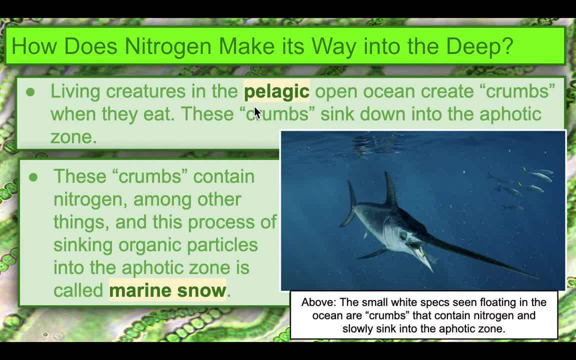 Okay, so we mentioned before the organisms that fix nitrogen In the ocean. they need sunlight, So down in the deep, deep ocean you're going to have animals that need access to nitrogen but there's no light. So how are they getting this fixed? organic nitrogen. 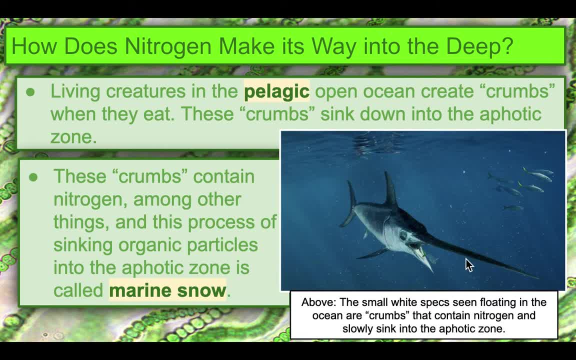 And the answer is this guy right here with the big schnoz. He's a messy eater. He likes to eat him some fish. Unfortunately, this poor guy looks like his next victim. He makes a lot of crumbs. Okay, this swordfish, all the fish that live. 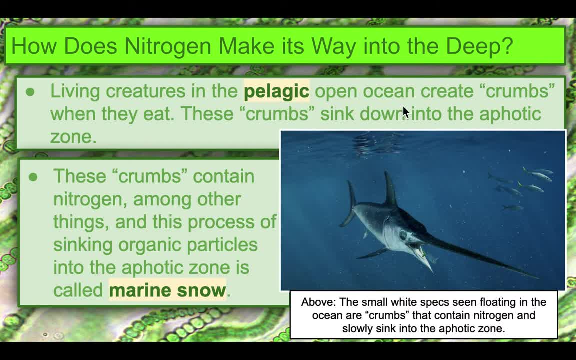 in the pelagic or the open ocean, they create a lot of crumbs. What I like to call them is crumbs, And these crumbs, these little white specks, you can see them. they all contain nitrogen, Nitrogen in the organic, fixed form that life can use. 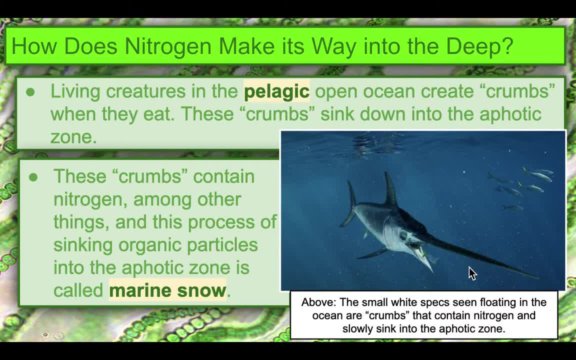 And these crumbs are going to sink down to the bottom of the ocean. It might take them months to get down there, literally to fall a mile and a half. It might take them a month or two to get down there, But when they arrive, the life. 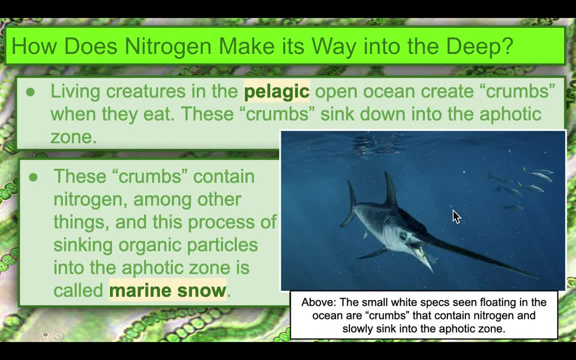 down there with the lights hanging from their heads and stuff, super excited to see this and they eat it. Okay, this process is called marine snow Because if you look at the particles they're white. It looks like snowflakes. So why? 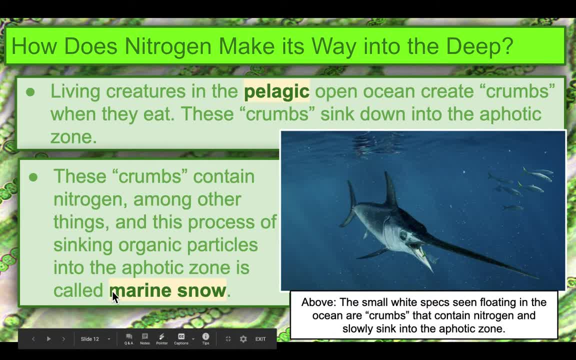 complicate things. I love it. I love it when things are not complicated. Okay, so marine snow sinks down into the aphotic zone, and that's how organic fixed carbon molecules make it down there, to those strange looking creatures with lights hanging off their heads, And that's how they're able to build their own. 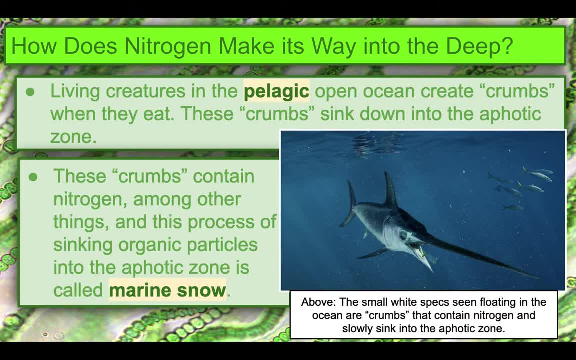 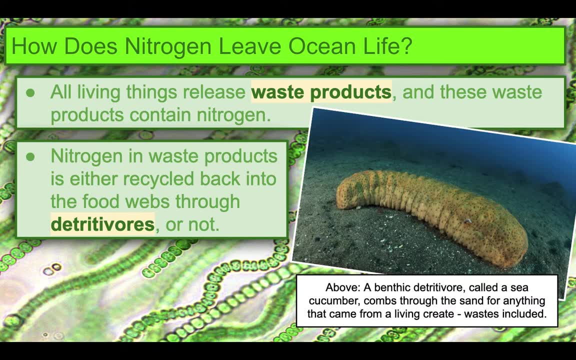 They're proteins and they make DNA and so forth. Okay, going back into the sunlit portions of the ocean, there's a lot of animals there too, and they're all releasing waste products. So where do these waste products go? 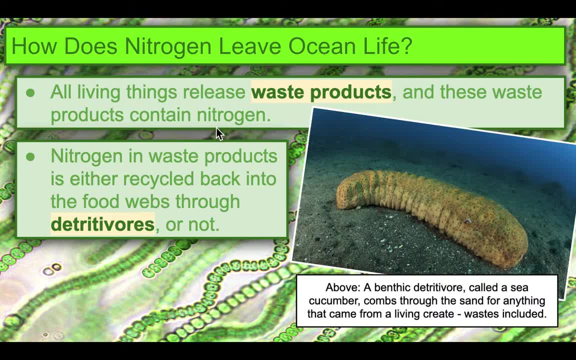 Because all the waste products are containing nitrogen, And if these waste products just kind of disappear, that is a huge source of nitrogen that is leaving life for good. That's not good, Because life needs nitrogen, So we have animals like sea cucumbers. 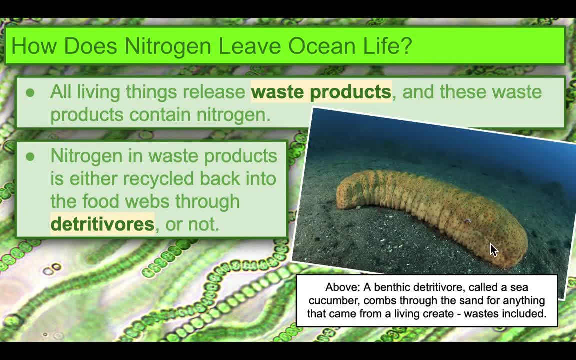 who are called the tridivores and their role is to crawl around and find all of this nitrogen that would have otherwise been lost to the sediments through waste products. You know animals dying. You know a dead fish might have died and fell over here a month ago and there. 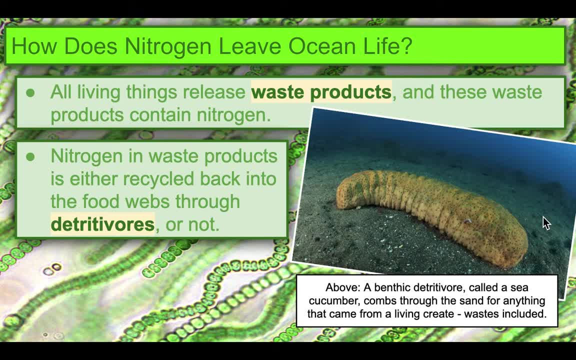 might be a whole bunch of nitrogen in the sand there and it would be locked away forever if it wasn't for the sea cucumber who would come around and eat that. So it's kind of a dirty job, but hey, somebody's got to do it. 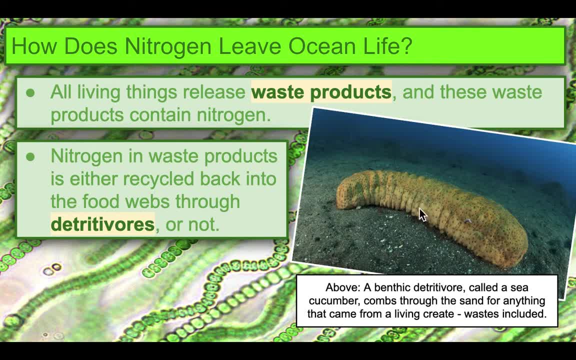 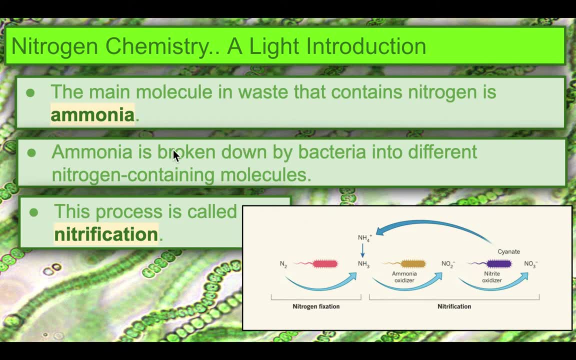 So here we have a very important animal responsible for recycling nitrogen back into the living, the living creatures. Okay, so the main molecule that wastes is going to contain is ammonia. Ammonia contains nitrogen, So this ammonia is. now we've started a game called hot potato. 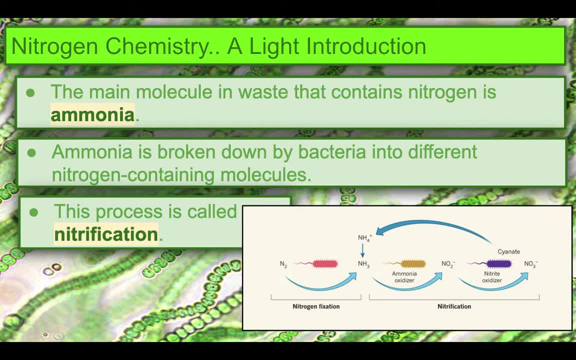 Pass the hot potato. Animals release ammonia. The game of hot potato begins, And this game of hot potato is called nitrification. So let's take a look at nitrification and the game of pass the hot potato. We're gonna just do a very light, quick introduction. 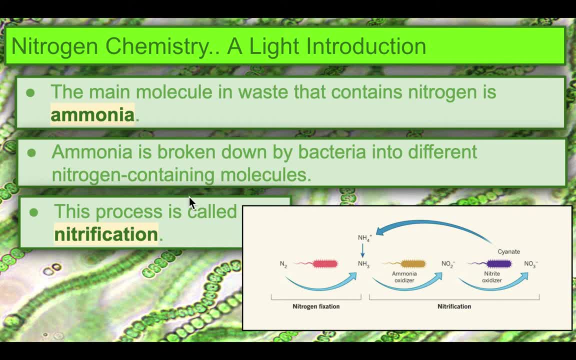 And what I'm about to show you for my students. I don't expect that you have you know this down completely, down pat. but this the process of fixation, nitrification and then the last part of the nitrogen cycle. that and understanding. 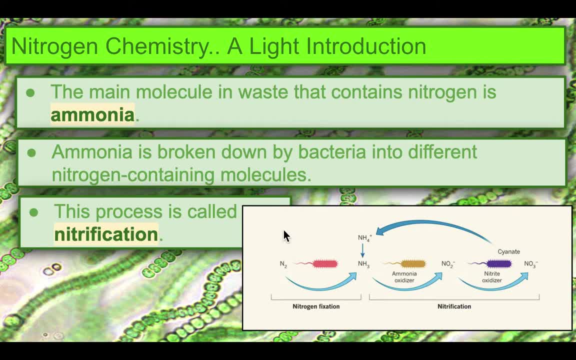 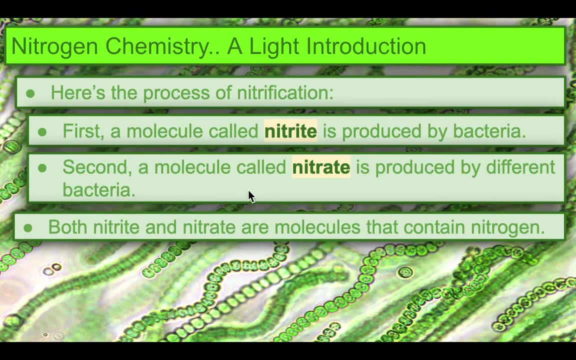 those three parts of the nitrogen cycle. that in itself is is very important. So what you're about to see, I'll go ahead and use the M word. It's not something I expect for you to memorize. All right, So the process of nitrification, or again pass the hot potato. 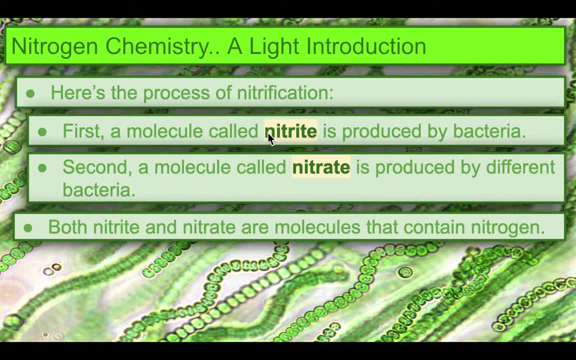 The ammonia bacteria are going to eat that ammonia and they're going to create something called nitrite. Another group of bacteria is going to take the nitrite As a food source and they're going to convert it into something called nitrite, And that's it. That's nitrification. That's the process of nitrification. 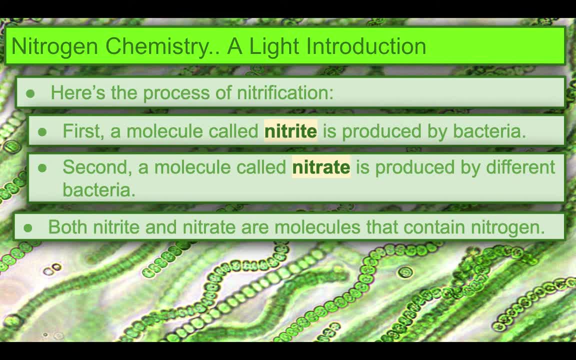 So let's stop, Collaborate and listen, Let's go back, Let's rewind. All right, We have learned about fixation, And now we have just finished learning about nitrification. So, um, Okay, Not so bad. There's one more part of that.